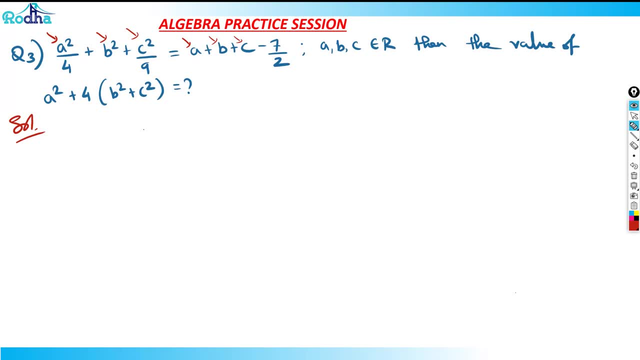 of b and a square of c and a single power of c. So what I can see by such kind of question that I should get the hint by now that basically I need to convert it into a form of property squares. actually. Okay, So by after that we can get the value of a square plus 4.. Basically you have the 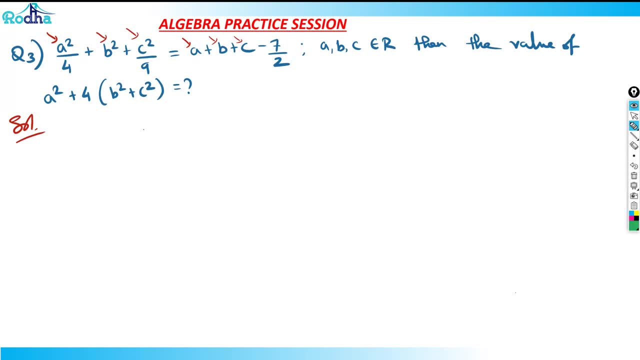 options also here, right? So we have the options. If I try to, if you get an idea, we were writing the options, right? So options are like 16.25.. Okay, We have 38.75.. Okay, Then we have 84.25.. Then we have 86. Then we have none of these here. 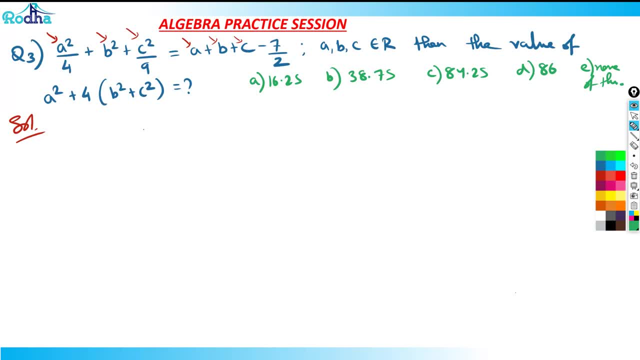 These options here, right, So that means we have to get the integer value here, Okay, So after you get this idea that I need to convert in the form of property squares here. So how are you going to solve it, guys? So you can just see like this: a square by 4 plus b square plus c square by 9.. Okay, 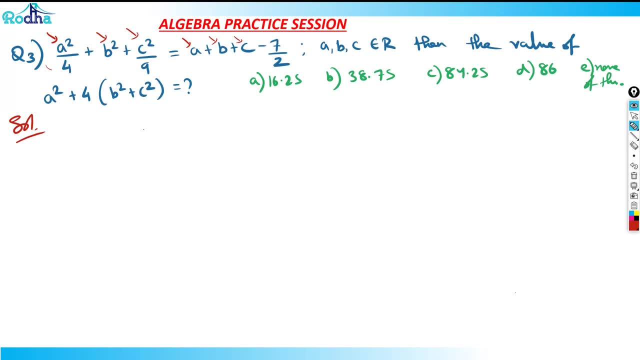 Now once a square by 4 plus b square plus c, square by 9.. So let me just try to write, write together the forms of basically combine the terms of a, b and c here. So I'll write a square by 4 minus a plus. 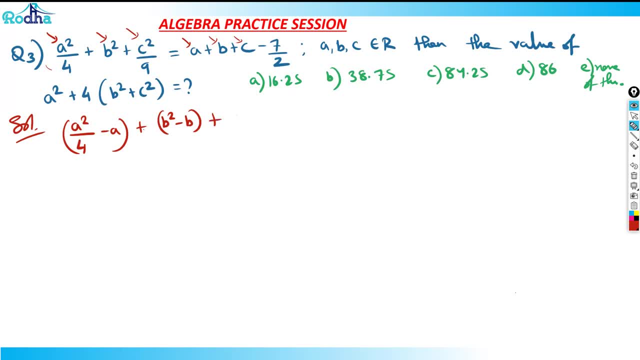 b square minus b plus c square minus c is equal to minus 7 by 2.. Okay, And now I got to this. I got to convert this in the form of a plus b plus, like perfect square form actually. Okay Now, so you can sense it here, right? So if you want to, 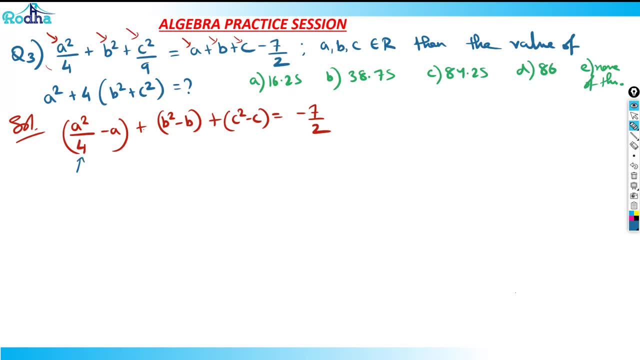 just try. you should be very, very quick at this. right, You can sense here that is a square by form 4.. I can write in the form of a by 2 whole square. Okay, That's something like x square, Now minus. 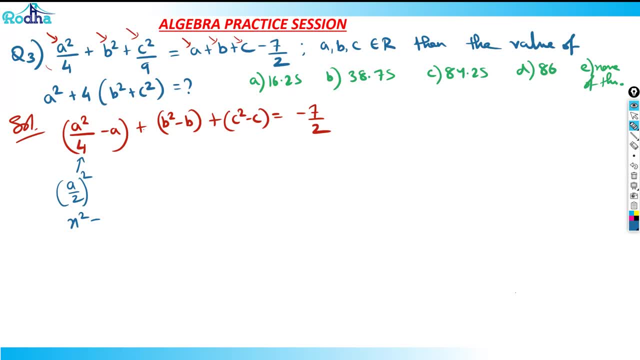 y square I want here. I don't have a y square. Single power means it has to be in the form of what It should be. go like, x square minus 2xy plus y square will convert in the form of what x minus y whole square. 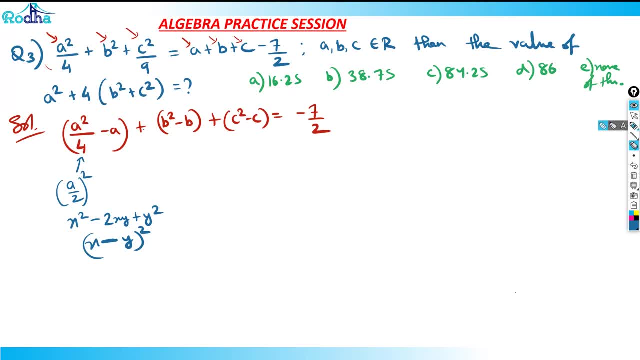 Okay, This is what it will convert, right. So if I, if I see this here, basically so a by 2 whole square now minus 2, again a by 2 here. So 2, 2 will get get canceled and I'm getting a here. Okay. 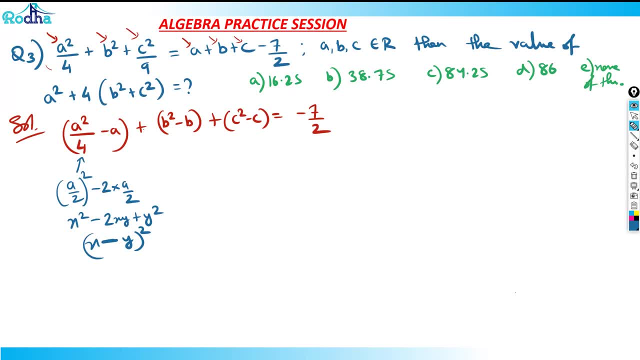 That means the y value should be actually 1.. So if y value is 1, that means plus 1 would do here right. Plus 1 square would do. That means y value should be 1 here. That means I can write simply: 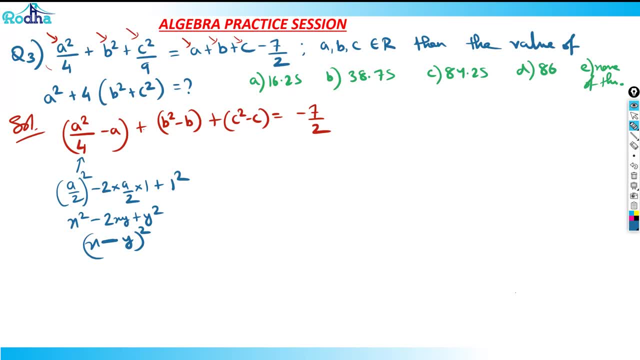 write this in the form of what? a by 2 minus 1 whole square. Okay, All of us should get this right. So now we can write this in the form of what a by 2 minus 1 whole square, So a by 2 minus 1 whole. 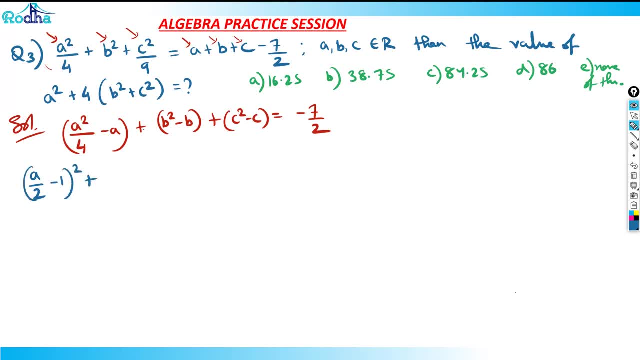 square plus similarly b, right, So b square is here. So for b term, what I can write here? So we have got 1 b and this should be again 2ab, right? So 2 into xy, So x is again b. and to get a b here. 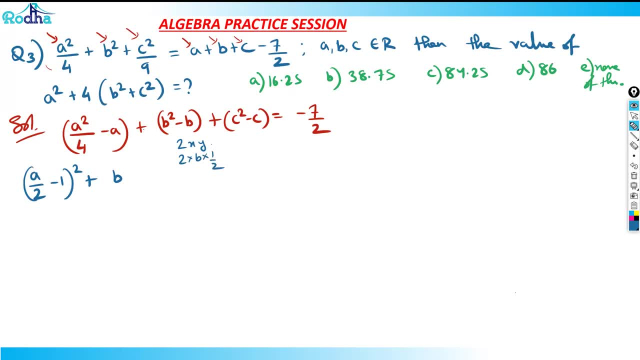 I need a half here. That means the y value should be half. now. That is b minus half whole square. Similarly should also go like C minus half whole square. Okay, Oh, sorry, C square by 9.. Okay, I missed it right. here Should be C square by 9 minus C. 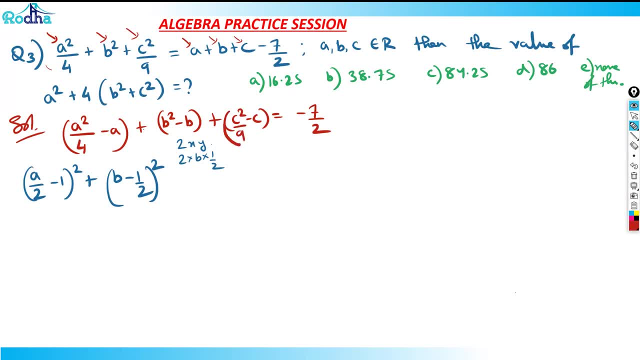 C square by 9 minus C here. Okay, Now look at these terms. right, Okay, So now, if you see here now- so basically now the last term- how it will go like: Okay, So the last term will go like this: So if you see here now- so basically now the last term- how it will go like: 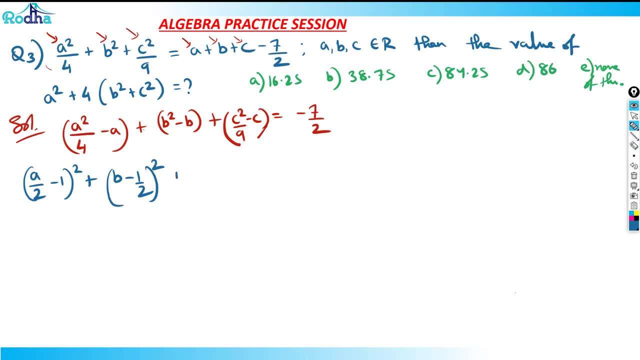 go like: yeah, plus now c by 3 and again. so this first term is c by 3. that is x square minus 2 into x- y. so you got that 2 into c by 3 here. you want to make it to c, right? so once you want to. 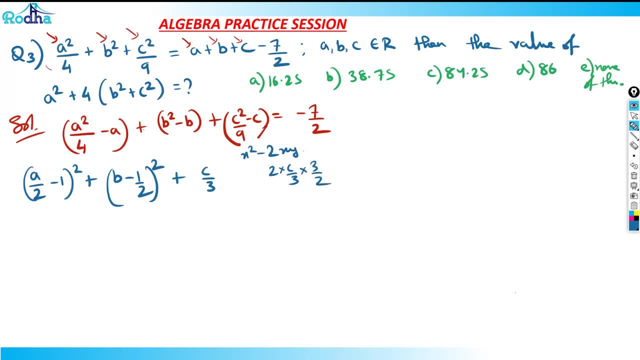 make it to c you got to multiply with what? 3 by 2. so you got to multiply with 3 by 2 to convert it to: so c, c. actually that means the y value should be 3 by 2 here. okay, if the y value is 3 by 2 here. 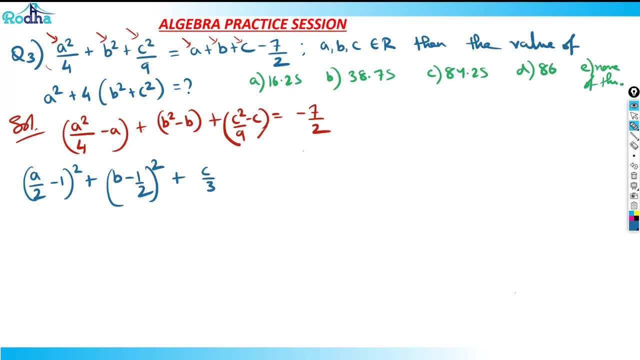 so let's say y value is 3 by 2 here, right, that means c by 3 minus 3 by 2, whole square. so c by 3 minus 3 by 2, whole square. okay, this is equal to what minus 7 by 2? this is equal to minus 7 by 2. 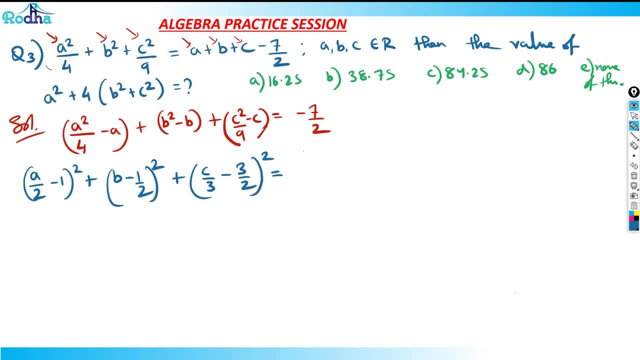 but here obviously i have added few terms here, right. so whatever i have added to the left hand side, same things i'll be adding on the right hand side. so whatever what i've added here, i've added extra plus 1. here i've added extra plus, i think, half square. that means i've added 1 by 4 here. 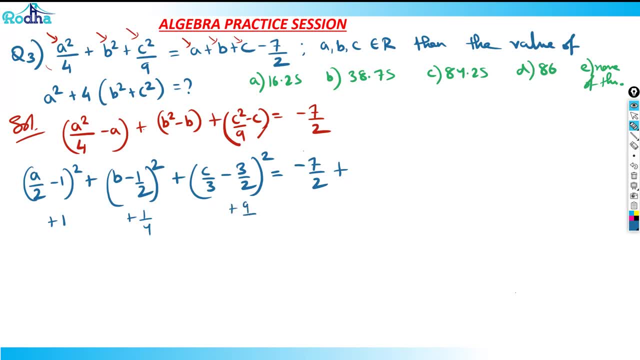 and i've added 3 by 2 square, that is, i've added 9 by 4 here. so 9 by 4 plus 1 by 4 is 10 by 4 plus 1. that is 14 by 4. that is 7 by 2. so 7 by 2. i've added this side, so 7 by 2, i'll add this side. 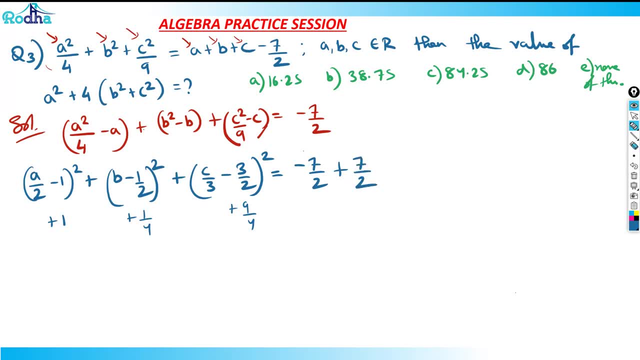 also, and now it converts to a beautiful questionnaire: okay, because this terms has become 0 and now it is actually sum of 3. perfect square is 0. that means a by 2 minus 1 whole square plus b minus half whole square, plus c by 3 minus 3 by 2 whole square is equal to 0. sum of 3 perfect. 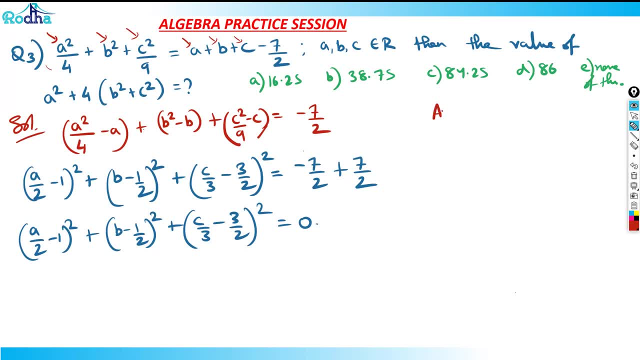 square is 0 perfect square: any. i know that any perfect square, any perfect square, will always be greater than or equal to 0, so any perfect square will always be greater than or equal to 0. so any perfect square will always be greater than or equal to 0, right? so in this case, what i can get here is: 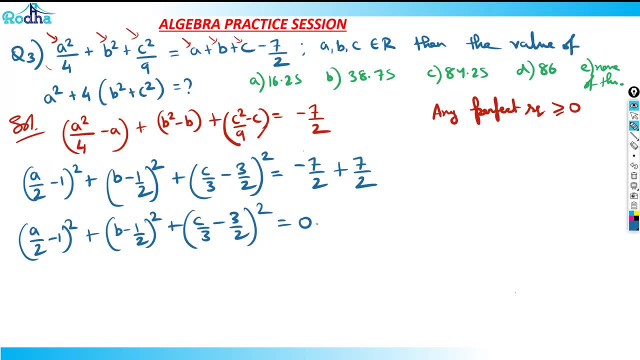 the sum of 3 perfect square is 0. that means all has to be 0. so that means if a ¯2 minus 1 is 0, that means a a is equal to 2. b minus half is 0, that means b is equal. 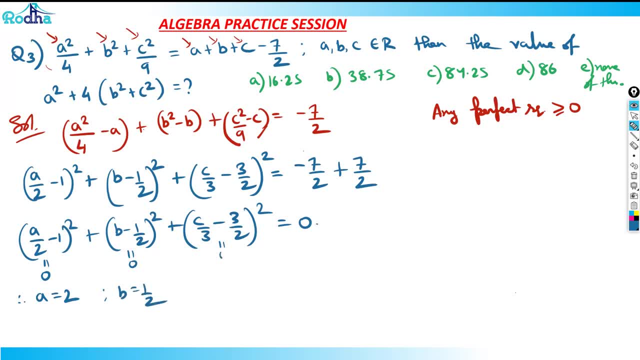 to half and c ¯ 3 minus 3 by 2 is 0. that means c is equal to 9 by 2. okay, so i was supposed to calculate the value of this part, right, this part. i was supposed to calculate only the 3x3 dxh, right? so this is make b n del cd, бs. everything else is equal to 0.. 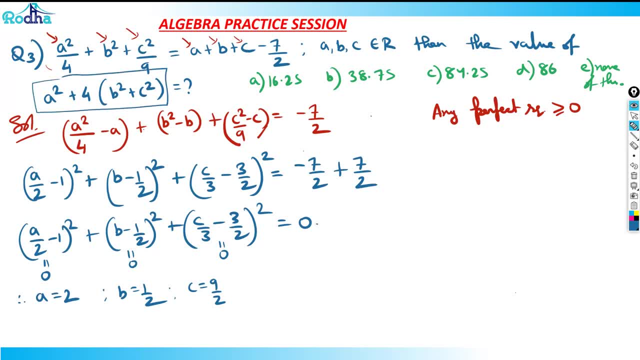 was. I was supposed to get the value of this part here, okay. so what is the value of this part now, guys? the value actually comes like this: now you can see here: a square plus 4 into b square, plus c square, that is a square, is 2 square, that is 4 plus 4, into b square plus c square, that is 1 by. 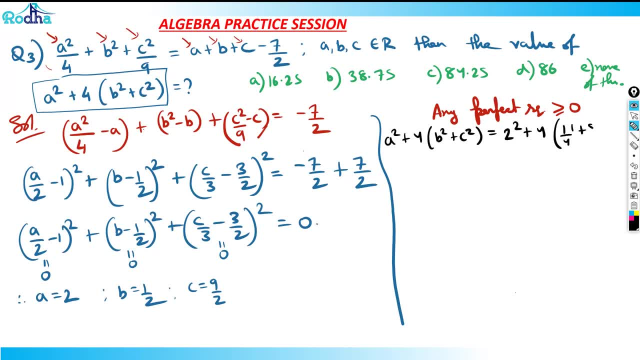 4 plus 81 by 4. 1 by 4 plus 81 by 4 here. okay, so now what I am getting here is that 82 by 4 is 40, 82 by 4, so 4 into 82 here, so 4. I am getting here 4 into this. 4 will get cancelled actually.